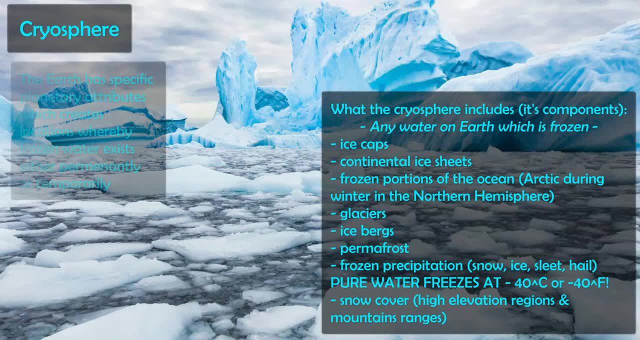 water into frozen water, which would be snow and ice and sleet and those mountain ranges that are certain altitude and elevation. then you have glaciers or glaciers, then you have ice caps and you have continental ice sheets and parts of the arctic ocean freeze over the winter months less so than there was. 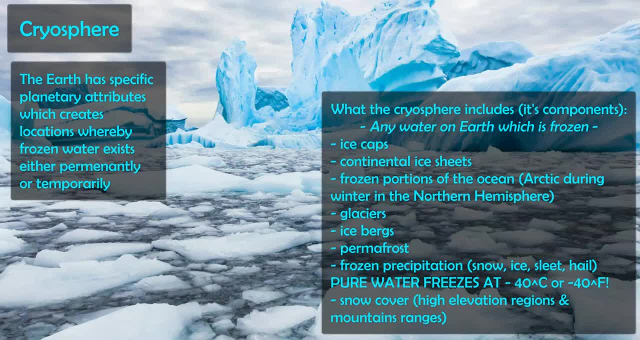 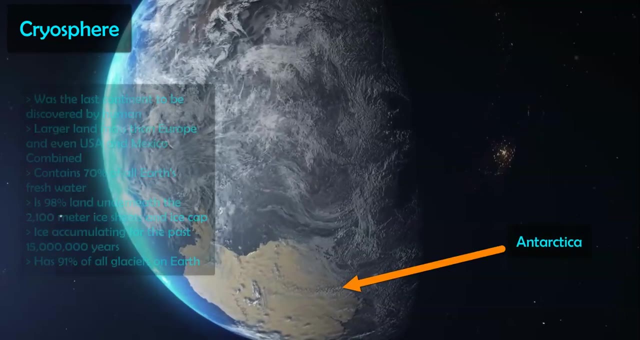 in previous centuries, and also looking at the frozen ground component, which is going to be permafrost, which happens again in high latitudes in the northern hemisphere, especially where temperature drops and temperature drops and freeze the soil subsurface. so we're discussing the cryosphere, one of the big topics discussed. 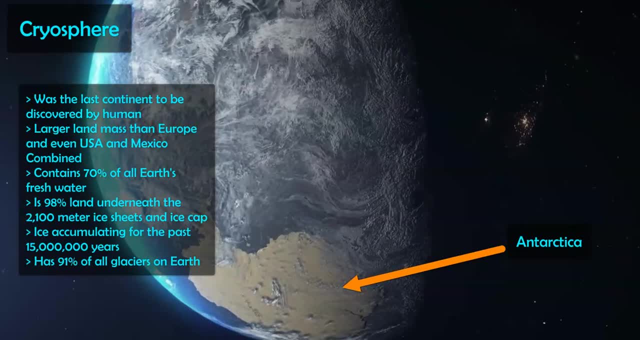 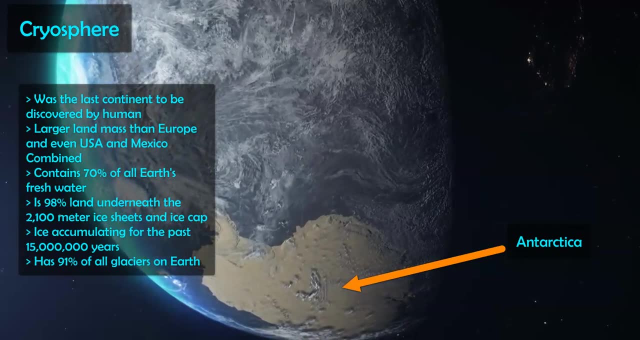 and what is amazing about it is the continent of antarctica, which was discovered apparently around 1820 and was the last continent to be discovered by humans, and obviously there's no one living there permanently. maybe in the past, maybe, but until it's been frozen like this with ice sheets and 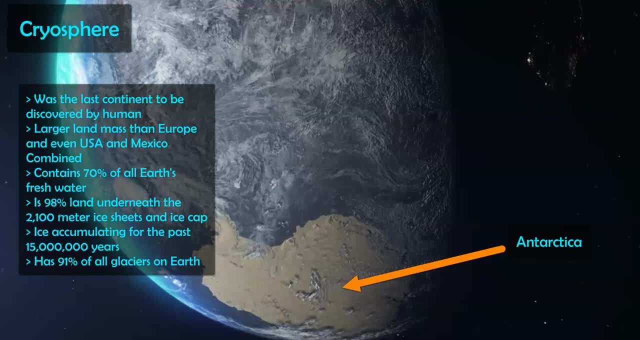 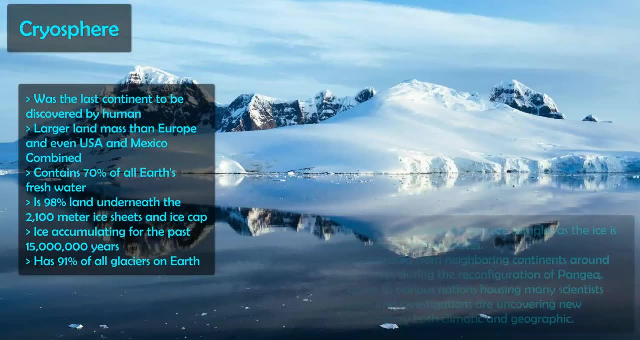 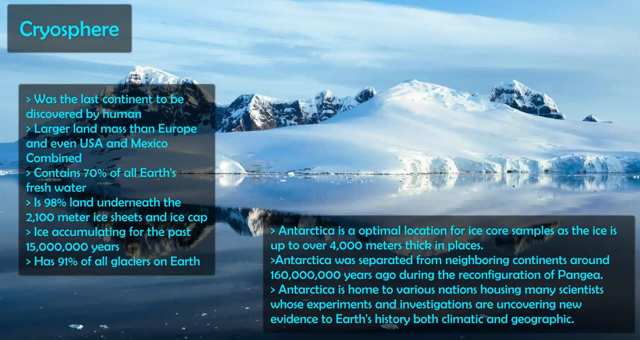 glaciers and glaciers for the last 15 million years- give or take a few million years- and has been separated from the other continents like africa and india and australia for the past 160 million years. so antarctica is an amazing place to do research on ice, on paleo, climate conditions and proxy pieces of evidence and isotopes of oxygen. 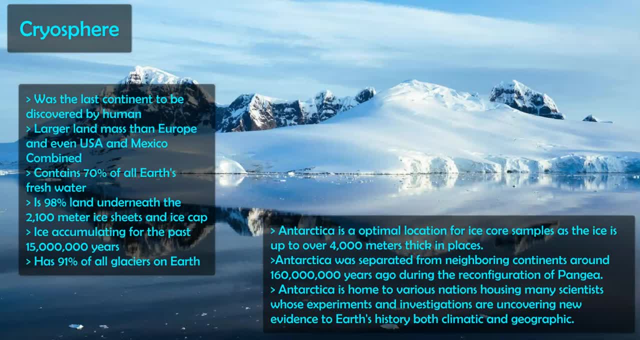 and nitrogen, other particles and particulates that can give ideas to scientists of how the earth was in the past and various ice ages and interglacias and other particles and particles that can give ideas to scientists of how the earth was in the past and various ice ages and interglacias. and 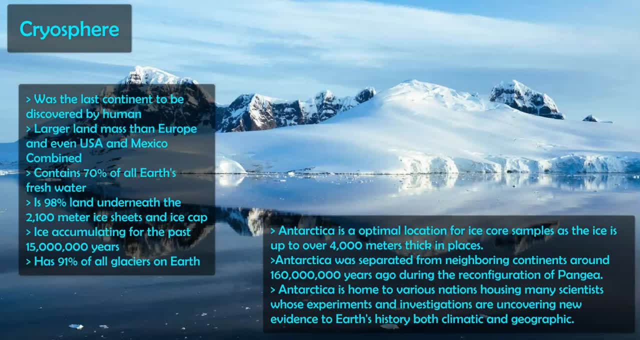 sacrificial and glacial periods and which are warm periods and cold periods in the earth's history. so no one really owns antarctica, but it does have various research bases from various countries like new zealand, australia, japan, america, england, germany have various scientists on there. 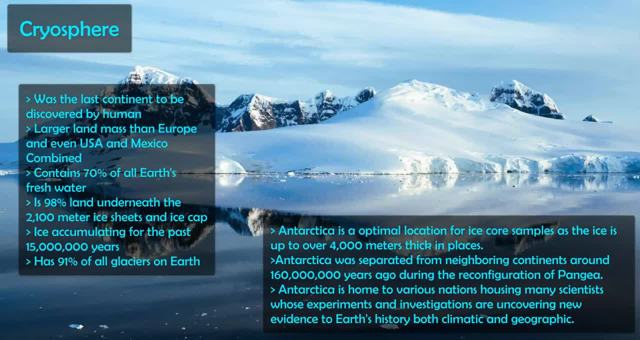 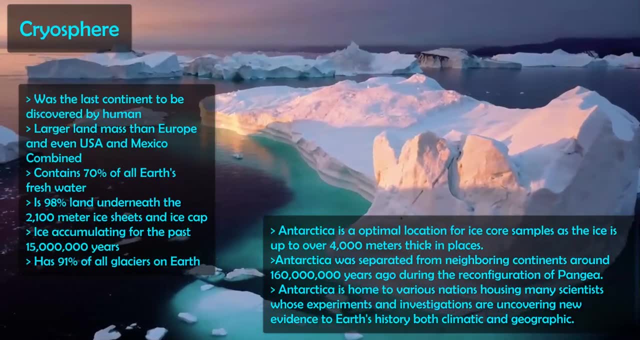 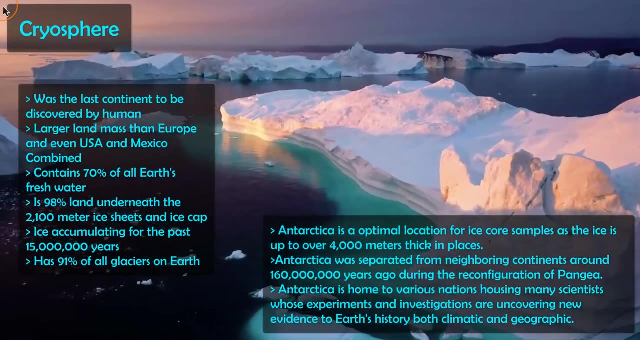 for a short time, but they generally leave during the winter months. so, in terms of the ice, antarctica has a thick ice cap of around. the average is about 2 100 meters thick, but the thickest parts around 4,700 meters thick and contains 90% of the ice on our planet, which also holds or contains. 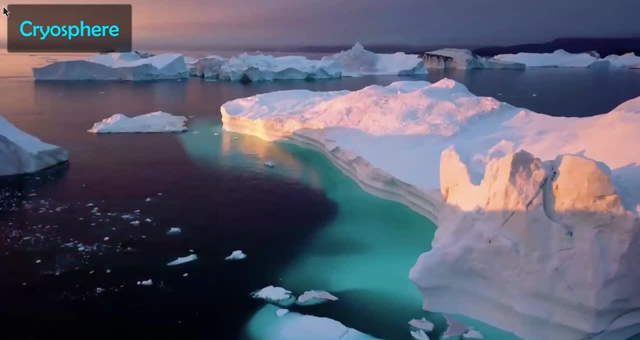 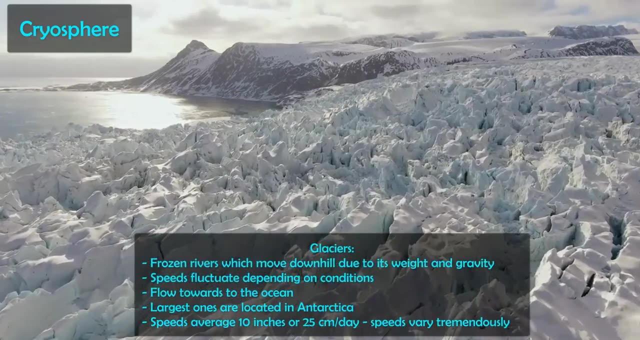 about 70% of our fresh water on this planet. So, with the majority of the water and the fresh water being trapped or contained in the ice around Antarctica and on Antarctica, you also look at glaciers or glaciers or frozen rivers, which are usually the exteriors of the ice caps, and you can 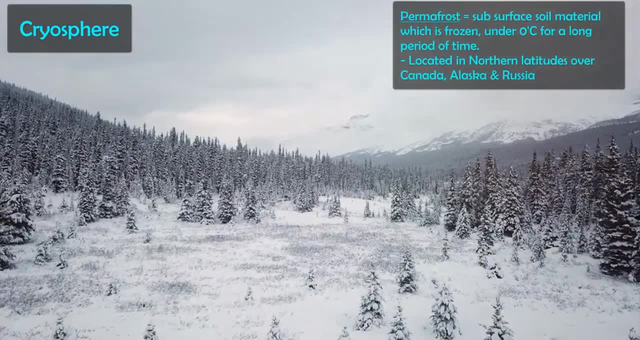 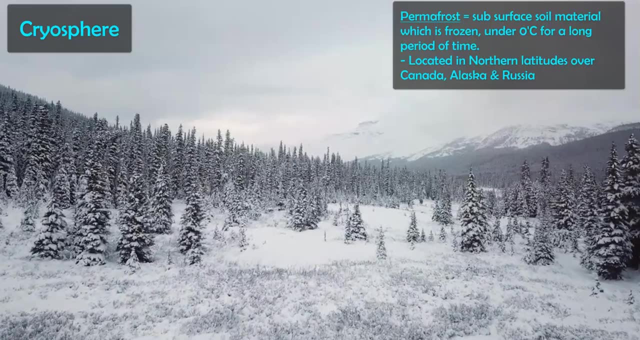 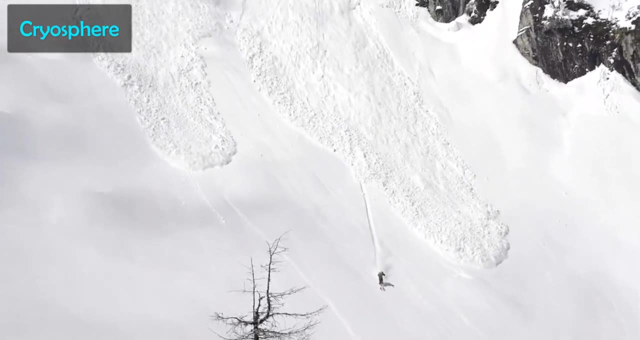 have them retreat and extend, based on the climate, So you can have permafrost in northern latitudes like this beautiful tundra and boreal forest landscape. So, in addition to the growth and expansion of ice sheets and glaciers or glaciers, or even the contraction and retreat of these, 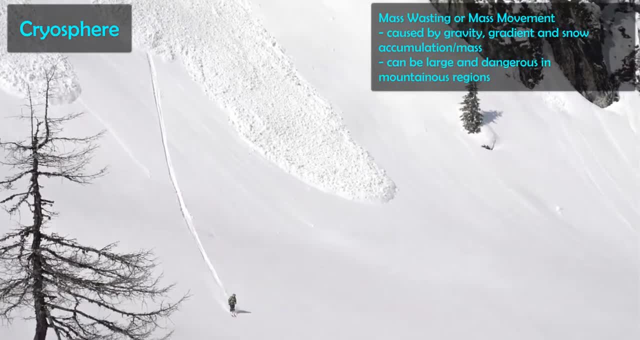 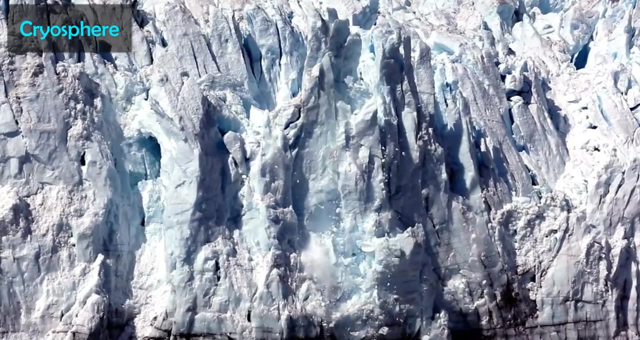 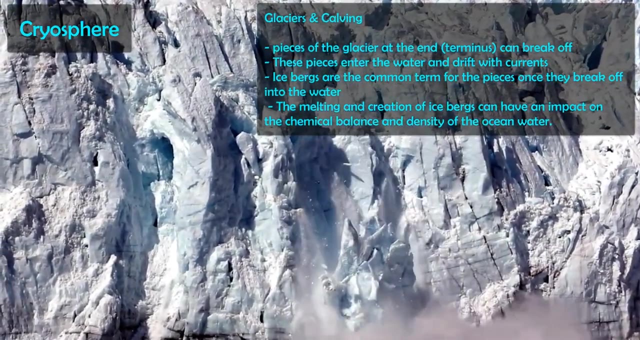 massive ice sheets based on climate conditions and temperature. we can also look at the mass wasting component, which in this case would be avalanches, And how they can move large amounts of snow and ice at one time, Also looking at the carving of glaciers or glaciers on the edge of the ice sheets, where the ice is going to break apart and fracture. 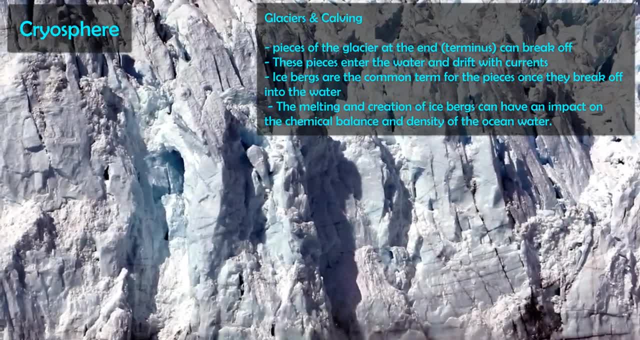 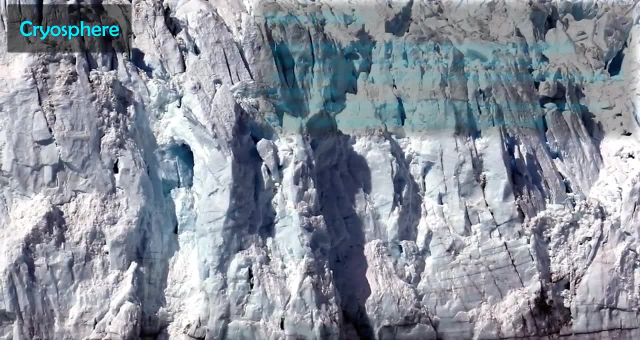 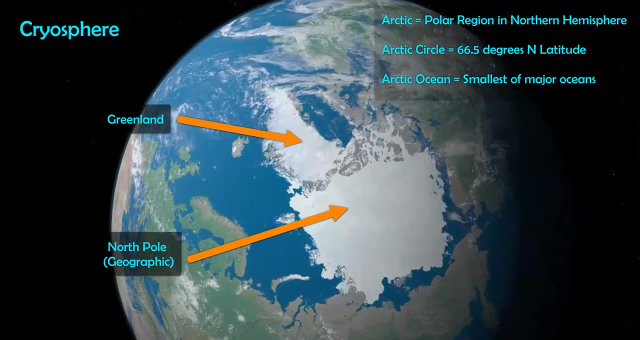 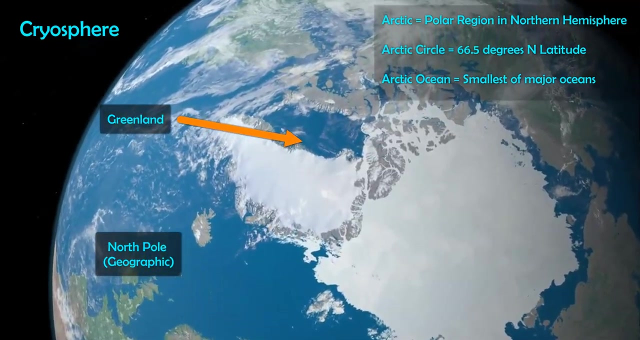 and fall into the water, causing various tsunamis and large waves, but also create a lot of these icebergs that will float in the water based on the currents. So we look at the cryosphere, We look at how the Arctic North Pole can freeze over the top part of the ocean, have a thin layer of ice over the 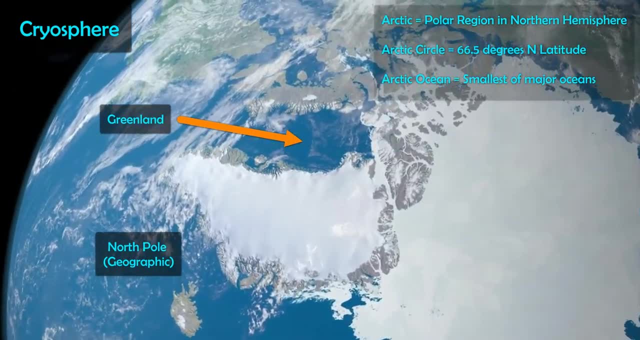 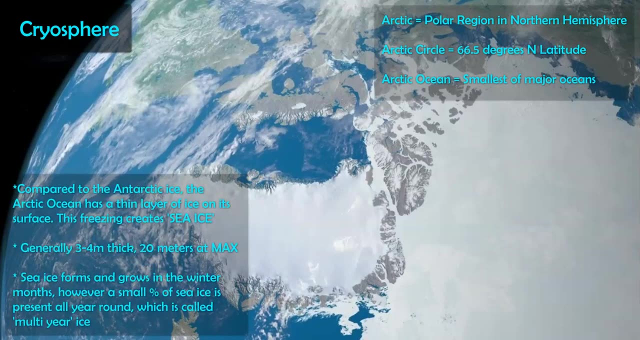 winter months. Now, this is the northern hemisphere, So we can look at the three to four meter average thickness of ice around the Arctic and Arctic Ocean, and at certain parts and certain times it can be as thick as 20 meters. So this is important because we can look at the extent of this ice and 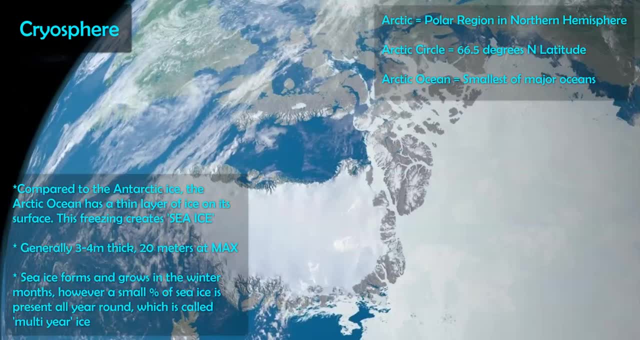 measure it and see the fluctuations with climate, with the climate, with the climate, with the different temperatures over a certain period of time, And looking at the ice ages and how ice can expand down through the northern hemisphere, through the land masses like Asia, Europe and 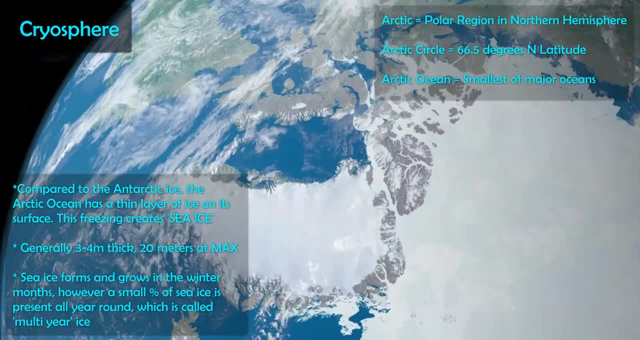 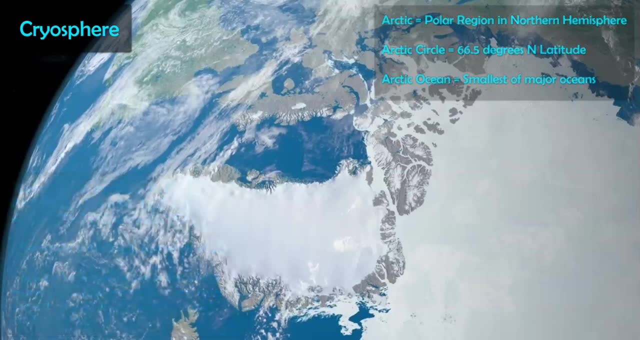 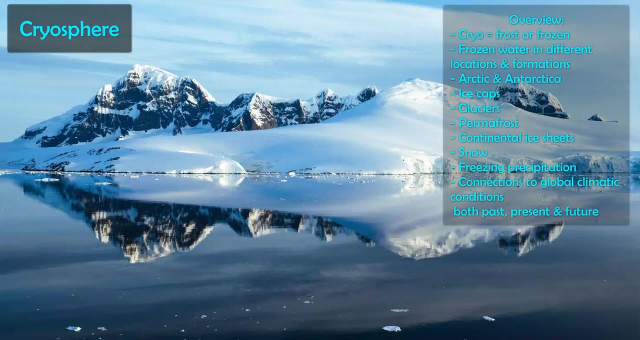 North America, through Canada and Alaska and into the United States and see how these historical ice ages have changed over time and the extent of the ice and how much land it covers. To summarize, the cryosphere is anything to do with frozen water, So anything in the northern South Pole.